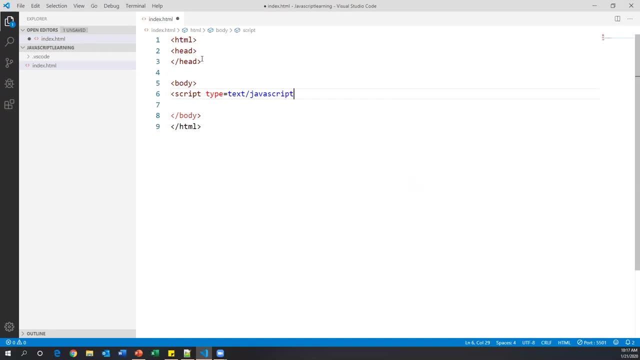 Right, So we need to specify what kind of text Script we are going to write inside the script tag And I need to refer SRC, where exactly my JavaScript file is placed. Right, So I will add the source here, SRC- later, once you created your JavaScript file. 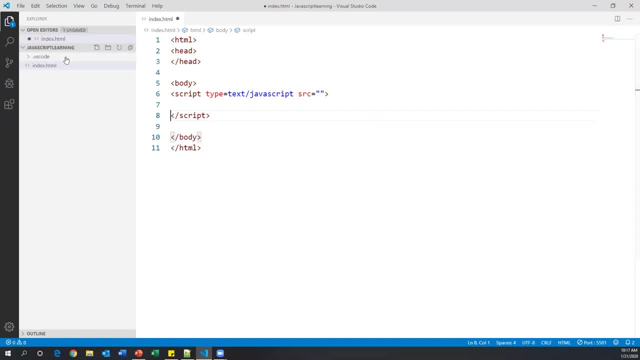 And for now just keep it like this. Now again I will create one more file, JavaScript file, This external JavaScript file I am going to create, And here I will say I will name it as JavaScript and variables: JavaScript and variables and data types. 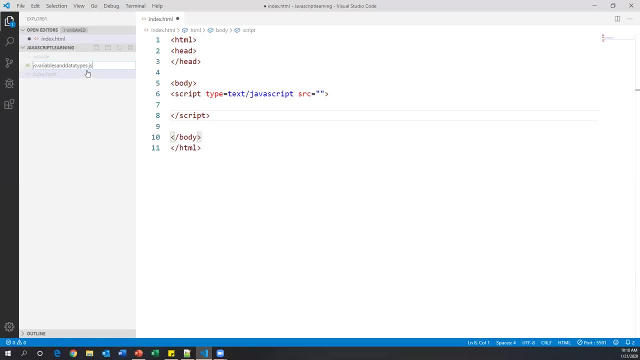 JS variables and data types: dot JS. The file extension is dot JS JavaScript file. So right, I have created another file. So one is HTML file, The other one is JavaScript file. Now, this particular JavaScript file I need to execute through HTML. 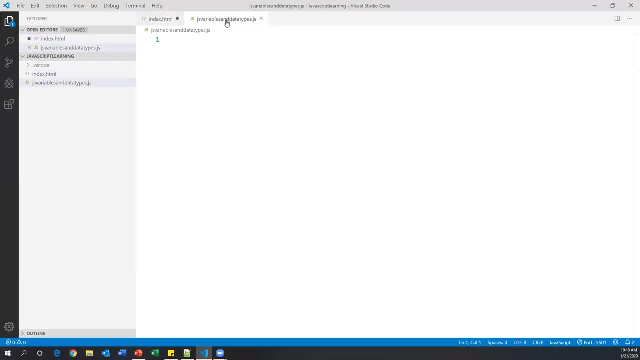 So here, SRC, we have to specify the location of JS file. Now let us get the location of JS file. Just click on this and copy relative path And go to HTML and page drawer here. So currently both HTML and JavaScript file are present in the same folder. 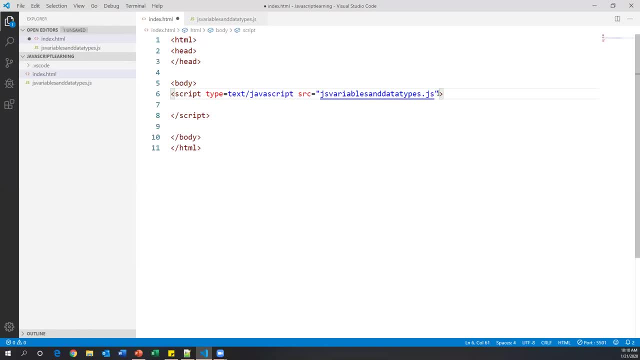 So I no need to specify the complete path. I can just specify the name of the JavaScript file. So done So whenever I run this HTML on my browser, So the JavaScript will be executed. So now I am going to write JavaScript inside JavaScript file. 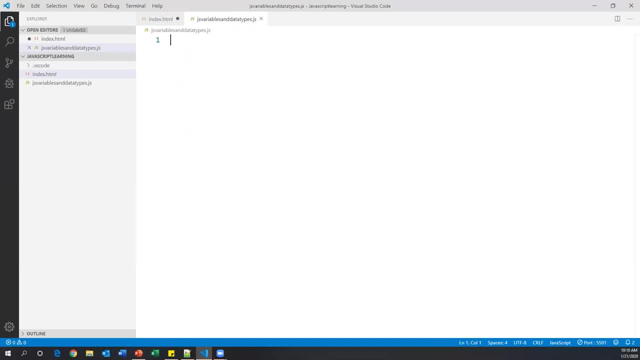 So first of all, let us start with the variables, So how we can Define or declare the variables. As said, three different keywords we have. One is var And other one is let, And then we have a const. There are three keywords are available. 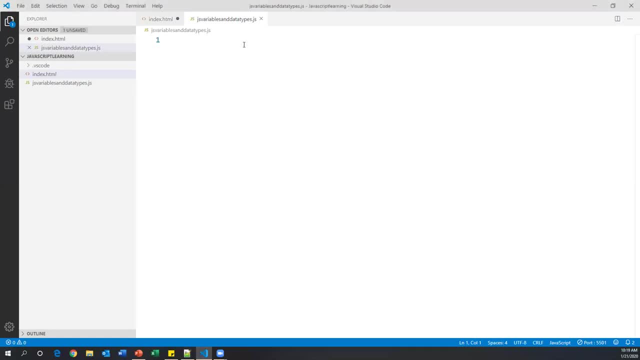 So first we will see how we can work with the var. So if you want to define a variable in JavaScript, You have to use a keyword called var, Let us say x. So this is simple variable And which doesn't have any data as of now. 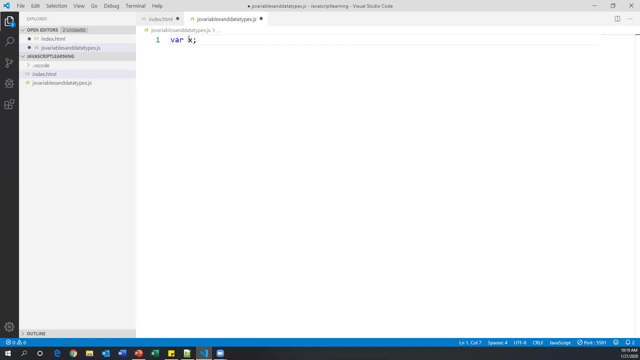 It's a simple variable. So as soon as I created this variable, It will allocate. It is occupying certain amount of space in the memory. Okay, So then I can assign some value into this. Now, x is equal to 10.. So x is a variable. 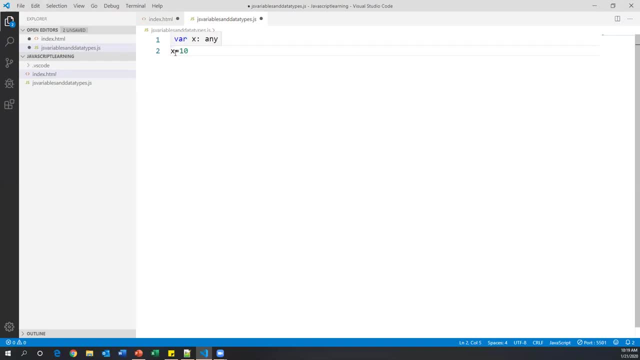 And the value of x is 10.. And similarly, I can also write these two statements in single line. And if you want to write in single line, We can say: var x equal to 10.. So we can write like this: Every statement will end with a semicolon. 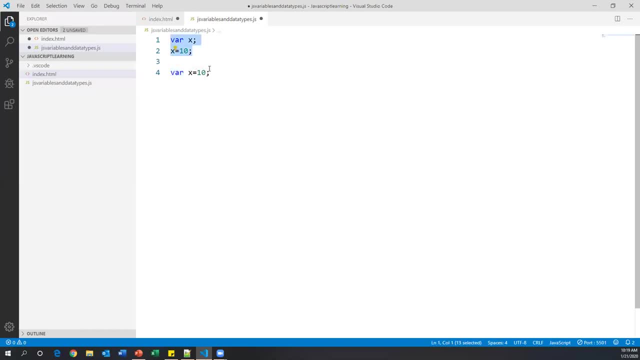 So here var x equal to 10. So we can also write these two statements in single line. So it is multiple lines or single lines. So this is multiple lines, Or this is a declaration part And this is an assignment part or initialization. 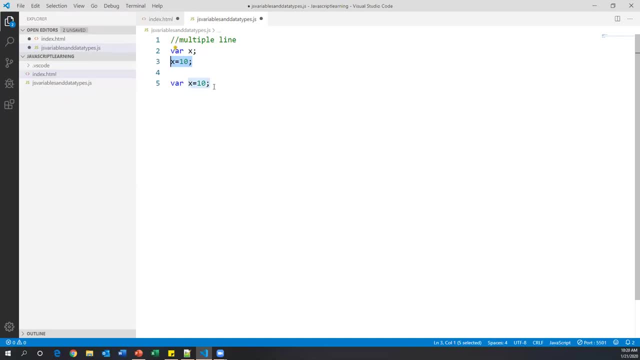 And here we have done declaration and initialization. Both we have done in single statement. So this is single statement, Which contains a declaration plus initialization, Declaration, initialization. So here this statement is declaration, Declaring the variable, And this statement is initialization. 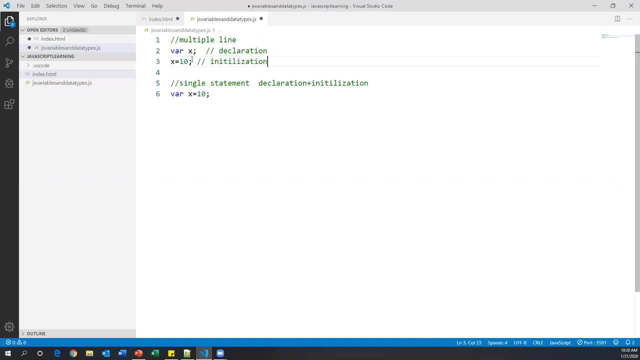 This is initialization. This is initialization Right. So we can, if suppose, if we have a multiple variables of same type, We can also define like this: There is another way. So, for example, let us say: var x equal to 100, comma y equal to 200. 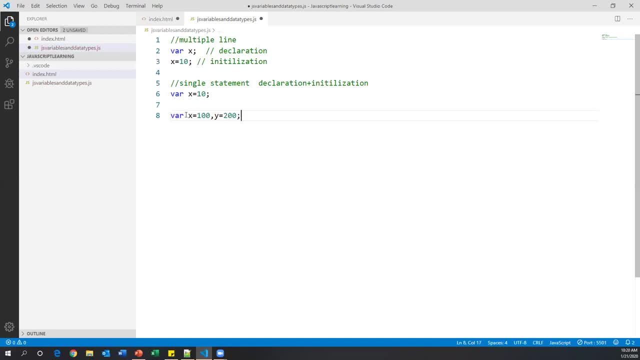 So we can also define the variables like this: If we have a multiple variables, We can specify the variable value. Again: variable and value. We can add any number of variables and values by separating comma. So we can also write a single statement and multiple variables. 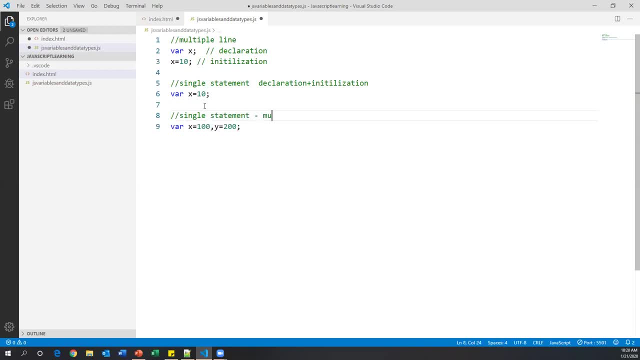 So here this is single statement, Single statement, multiple variable, And these variables can be different type. also, We can store different type of data, like numbers, decimals, strings, characters, Any kind of data we can store in this variables. So this is another way of creating the variables. 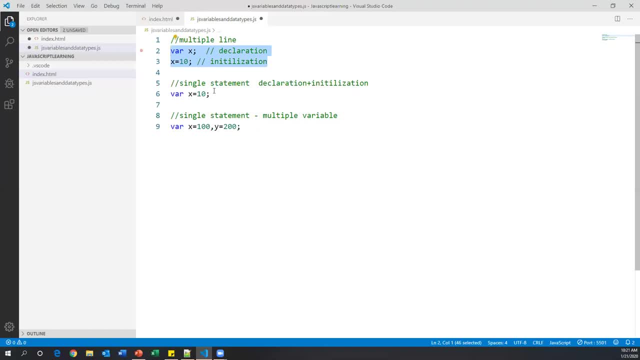 So declaration, initialization, we can do in multiple statements, Or we can still do in single statement, Or, if we have a multiple variables, We can specify within single statement. So this is how we can define the variables: by using var keyword. Now let us print these variables. 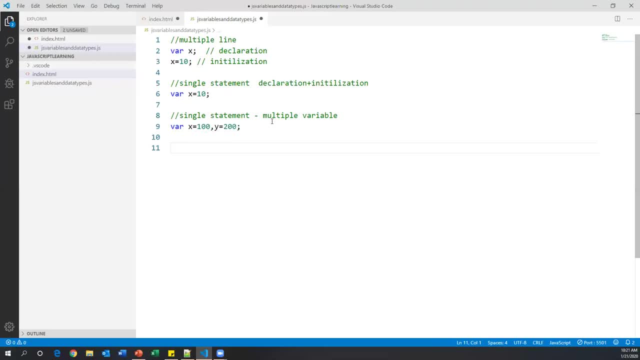 So to print these variable values We can use two different ways. One is we can use document dot write, Or the other one is console dot log. So first of all let me use, let us say, document dot write. So what this method will do is 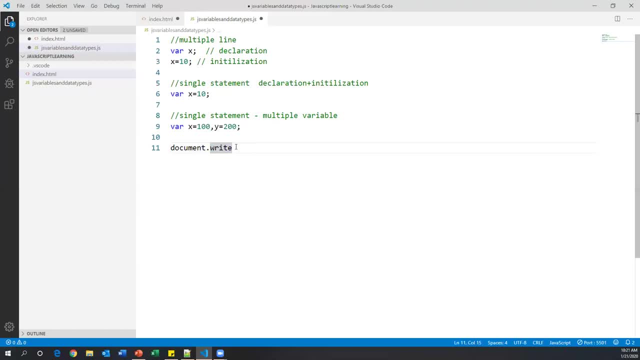 Document is an object in which write is a method. So I am just printing the value of x, So the value of x will be 1.. And I printed on my browser Because, as I said, document dot write, So let us save the file. 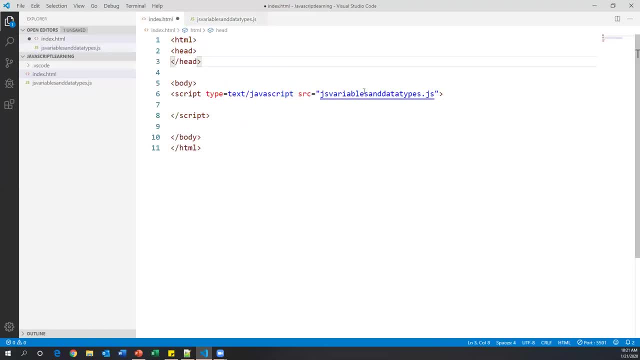 And which is already specified the location of my javascript file in html. Now we need to run this html on our live server. So in earlier session we already installed live server, Just we need to open this html. Right click. open with live server. 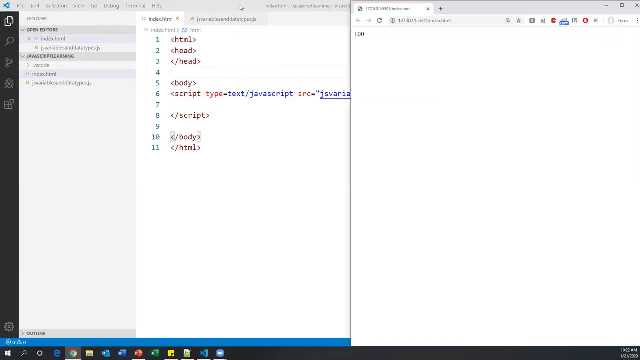 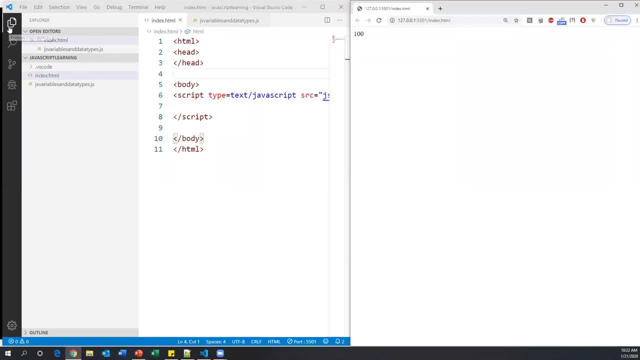 So automatically, the live server will be launched here. Now you can see, And this is my live server. This is my live server And this is my javascript. Let me just compress this. Now. my html is running on my browser. Now you can see here: 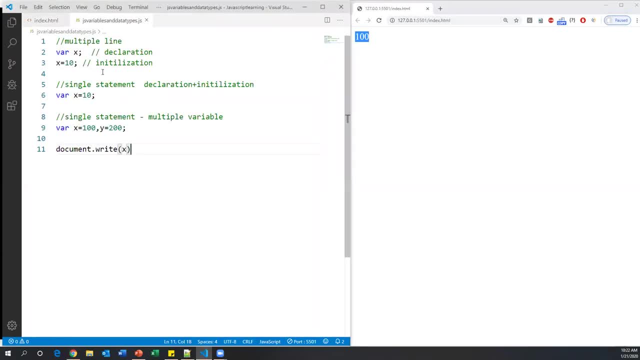 This is the value we got, So current value. So in the javascript, So this is the latest value of x 100 is printed, So I can also print. I can also print this one. Let us say I want to print the same output in my console window. 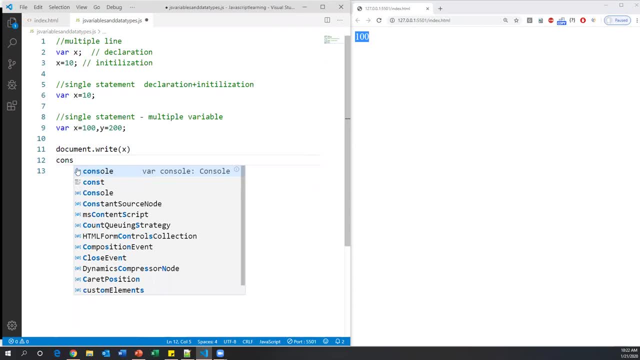 Then what I can do is I can simply say console, Console, dot, Log, And here also I can print value: So x value Now, save it. Now. apart from this document, You can also get this value in our console. So where we can get the console? 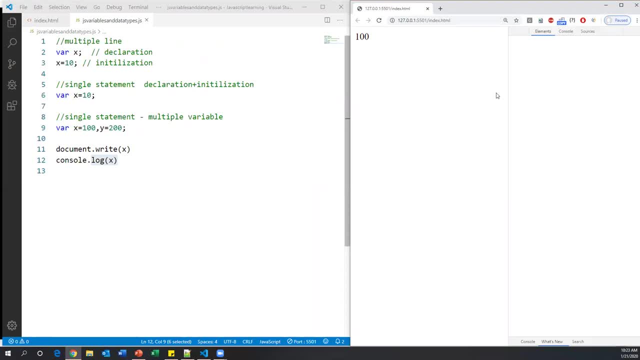 In our web page. Just right click on inspect And you will see A new tab called elements And beside that you can see console. So here you can see the 100.. So when I use document dot write method, You will see the output on your web page. 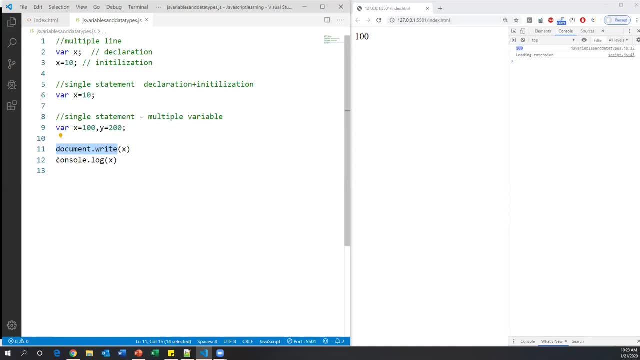 That is a document, Html document, And when I use console dot write, When I use console dot log, The same output you can see on the console window on your same browser. So here you can see 100.. Okay, So this is a way we can define the variables. 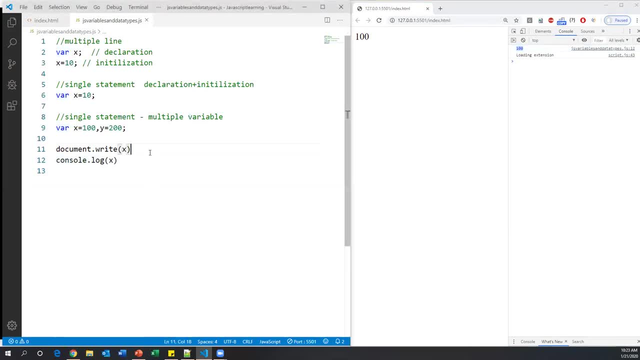 By using var keyword. Now, the same thing we can do by using let keyword. So let is the latest one. So most of the times we use let keyword, We can also go with let, But there is a small difference between var and let. 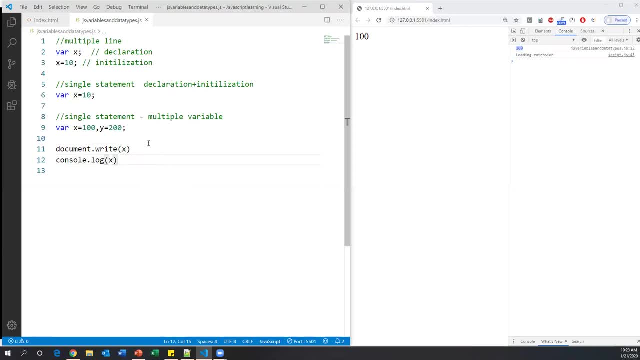 So first of all, let us see how we can work with the let keyword. So what I can do is I can just comment all these things for now. So now we will see how we can work with let keyword. So the same variables we can define with let. 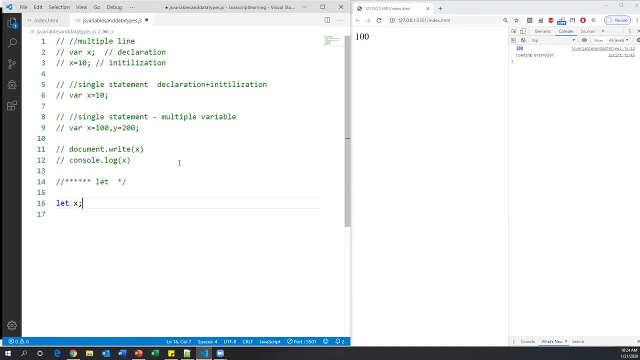 So here I will say let x. So this is just a declaration. Now I can assign some value to the init, So I will say 100.. And you can also assign some string data. So in the double quotations I will say welcome. 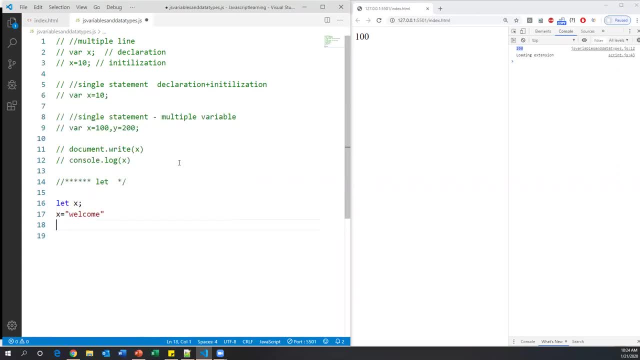 Okay, So now I can just print this. So let us say: if you want to print this Again, we can use either documentwrite or consolelong. So let me write the consolelong of x And then semicolon Right Now, save it. 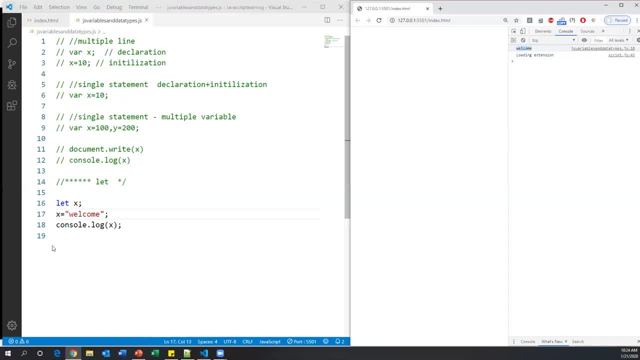 Now you can see in the console window you can say welcome. So here I have defined the variable, Then I have assigned the value. So this is again declaration. This is called declaration And this is called initialization. We have initialized the value. 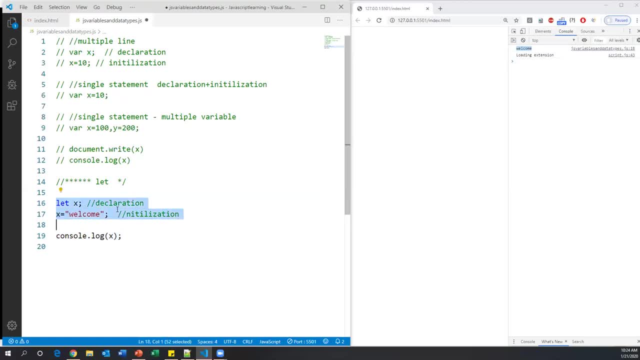 And then we have printed the value Again, we can write the same two statements in single line. So here multiple lines. we have written: These are multiple lines. Here declaration Variable. declaration is different And initialization is different. Initialization is different, Right. 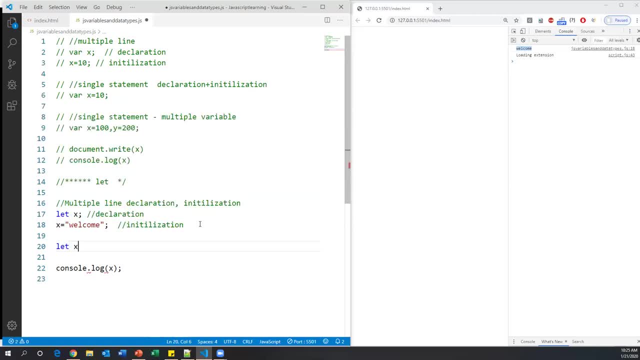 But now I can write both things in single statement. Let us say: let x equal to In the double quotations, I will say: welcome, It is a string value, Semicolon. So instead of writing two statements, I can write a single statement. 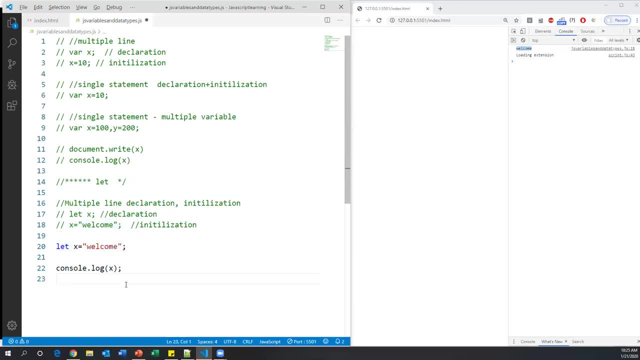 Let x equal to welcome. Now I am printing the value Now save it. Now we got the same value in the console window, Right? So this is single statement. Single statement which includes declaration plus initialization, Initialization. So this is the way we can use let keyword. 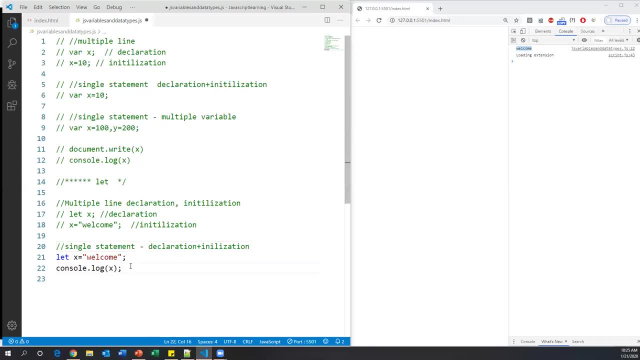 And similarly, if you have a multiple variables, You can also define multiple variables. So let us say, multiple variables in single line, Multiple variables in single line. You can say like, let me just comment this, And multiple variables if you want to define. 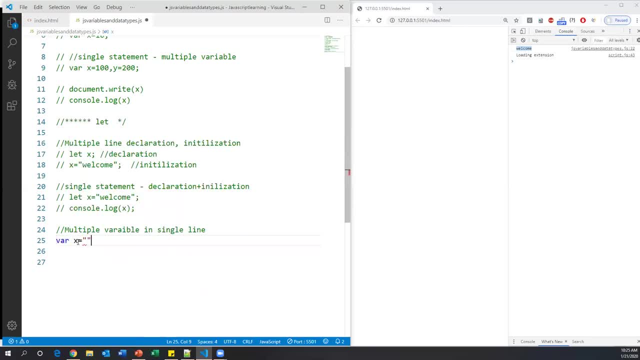 I can simply say: var x, equal to welcome. So this is one variable. And you can separate with comma. Let us say y, equal to. You can say: specify number, Perfect. So this is one variable. This is another variable. Now let us print this: 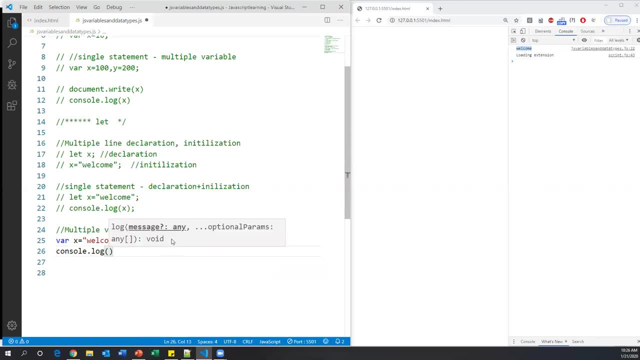 I will say console dot log And I will print x value first, And then again console dot. I will say console dot Again. one more statement: Console dot log And I will say y. So here x is a string and y is a number. 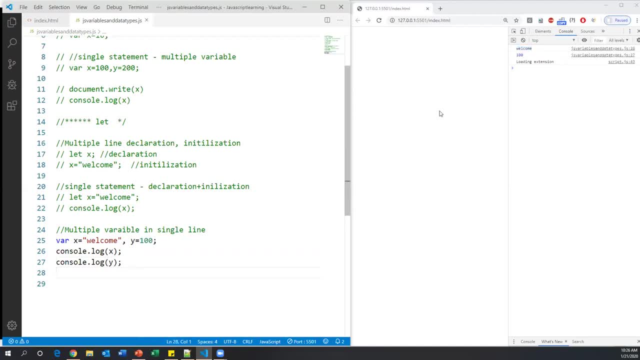 So let us execute these two statements, Save it And then automatically that will be affected on your console dot window. So welcome is an output of the first statement, And the value of y is 100. So you can also specify the multiple sets of data in different variables. 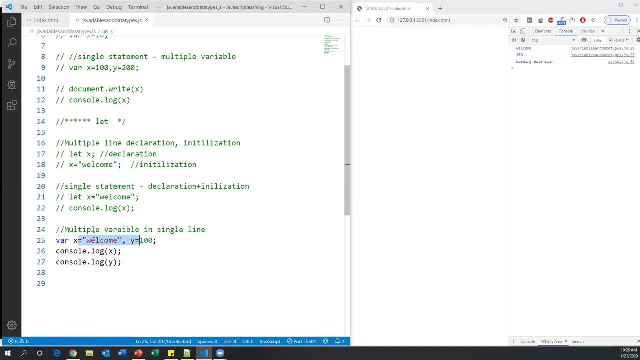 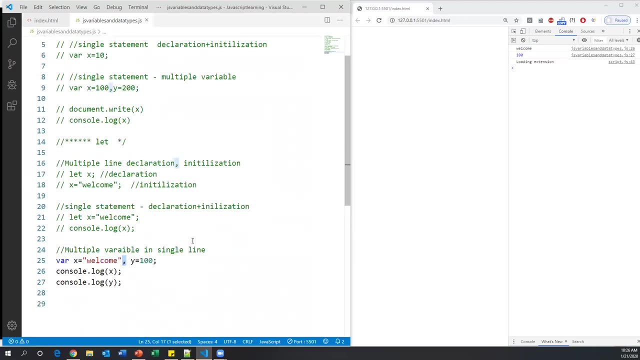 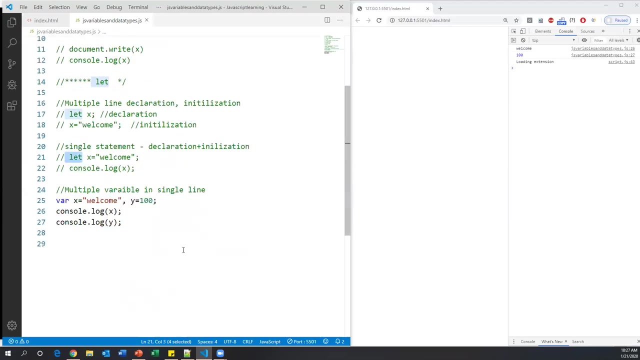 So here we can see multiple variables we have created within single line by separating comma Right. So we can define the variables by using var keyword or we can use let keyword. So these are the two keywords And there is one more keyword is also there: const keyword. 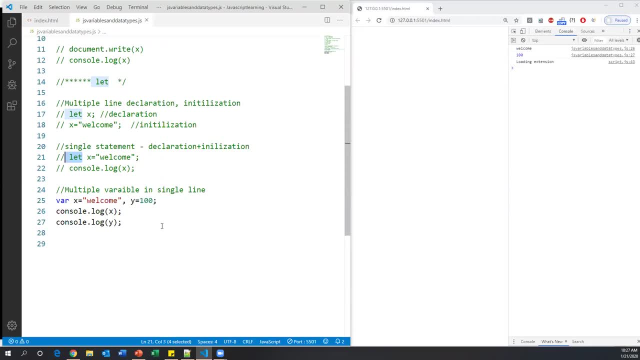 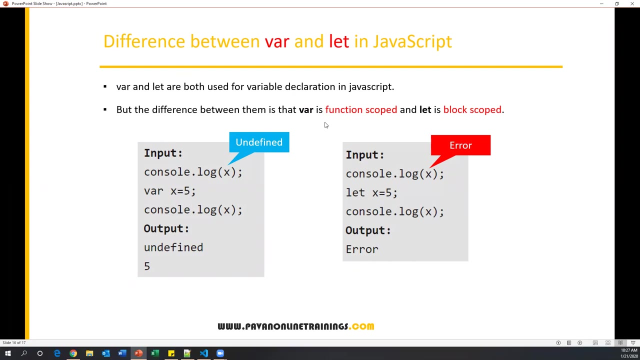 But before discussing const keyword, Let us understand What is the basic difference between var and let keyword. So I will show you one small difference. So the difference between var and let is In var keyword. var is basically function scoped, Whereas let is block scoped. 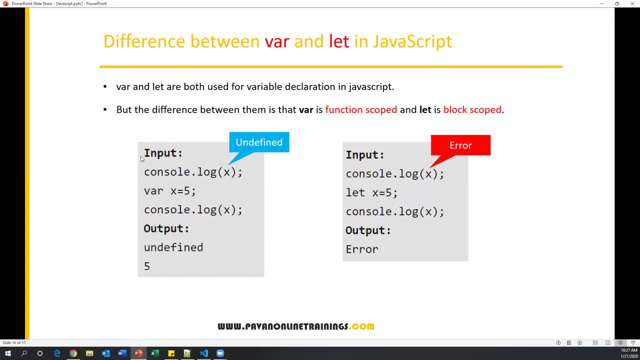 What is function scoped and block scoped. So let us see this example here. I have directly printed x value on our console, Let us say console dot, log of x, But by the time I have not defined any value for the x, I am directly sending the value of x to the log. 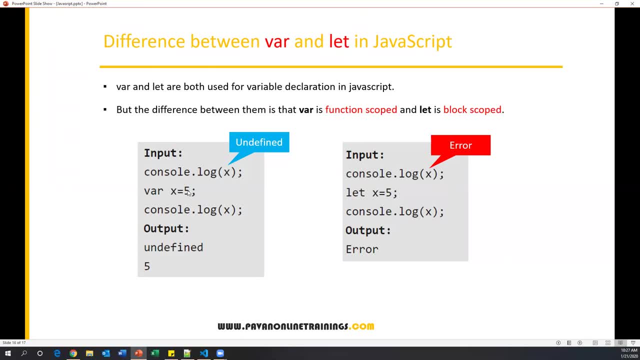 And after that I have defined the variable here, var x equal to 5.. And again I am printing this, So this code will give you the first output of this statement is undefined. The second output of this statement is 5.. Because here x is value 5, we have defined 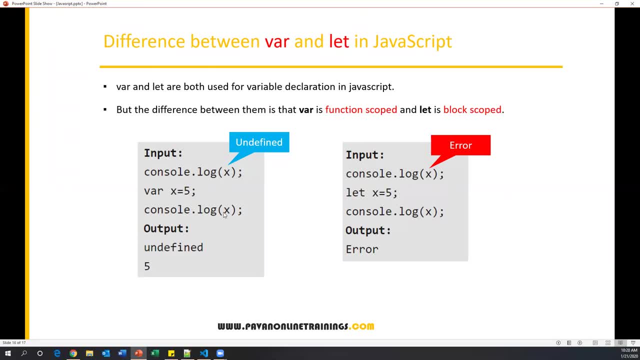 So the second log statement will print 5.. So why? because here x is not defined so far, So it is just giving undefined. But when you use let keyword, then what happens? The same code I have written here by using let keyword. So when I use let keyword, let is a block scoped. 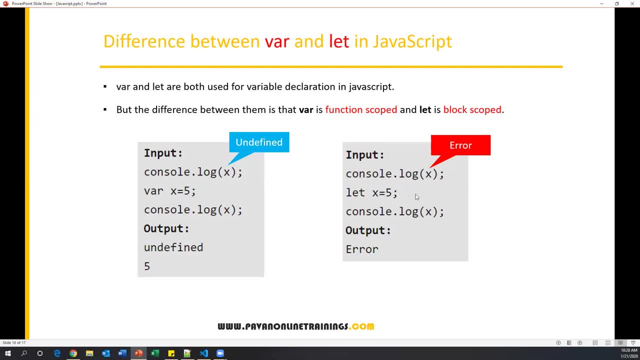 So, before this, define the variable let x equal to 5.. Before that, if I use console dot log, this will throw an error. This will throw an error Because this is let is a block scoped. That means from here, whatever statements we have created below the let. 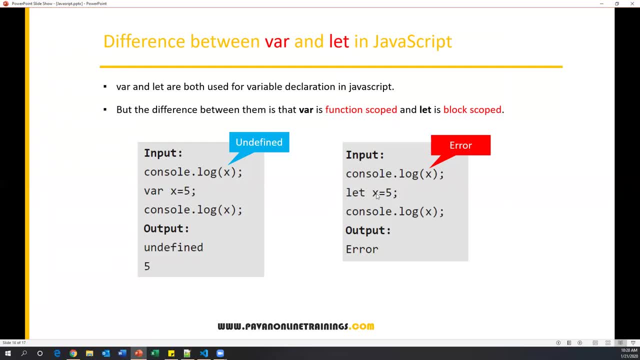 All the statements can use this variable x, Because this is block scoped, Whereas function scope- this is var- is a function scope. Function scope means that variable we can use or we can refer anywhere in the function, But let is a variable which we can refer within the block. 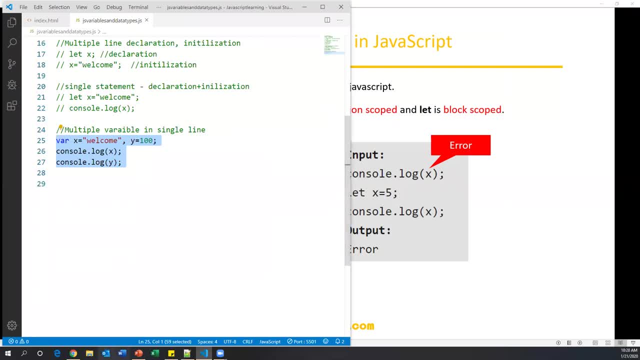 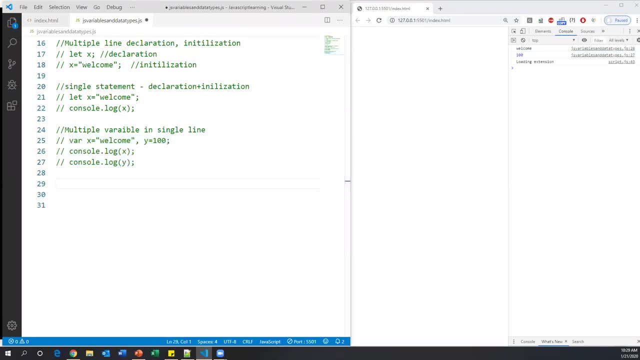 Let us see, practically, let us go to visual studio again. So let me just comment this. So now I am going to write a script here. So difference between var and let, Var and let. Difference between var and let. Let me open the comment. 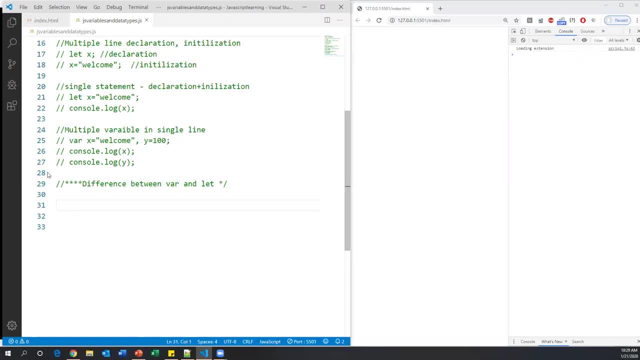 So difference between var and let So let us write it here. So first of all I am directly printing, let us say console dot write, So console dot log, And directly printing x. So so far I have not defined any value for the x. 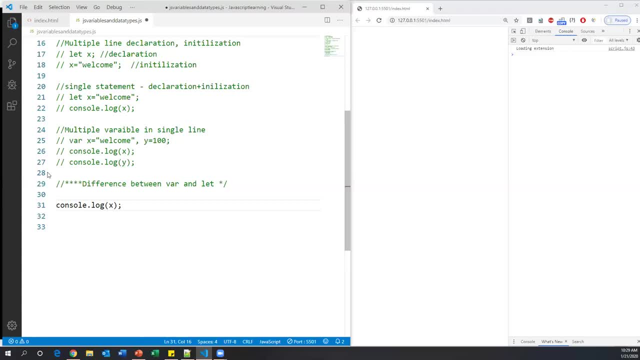 Not even variable. right, I have not defined any variable as x, But directly. I am directly Sending the value of x to the console Without having any declaration. After that, I will use var keyword. Observe this. I am using var. 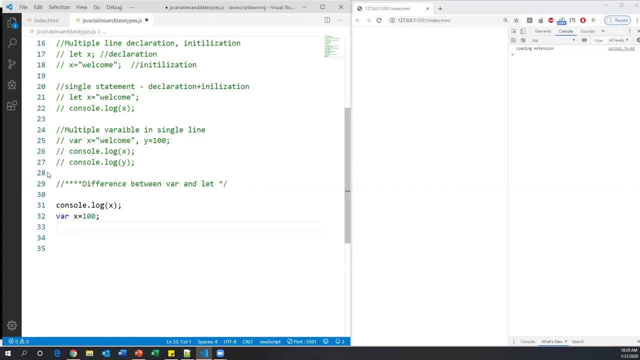 var x equal to. I make it as a hundred Again, after making x value hundred. Then again, console dot log x. Just print the value of x, Just as these statement I have written. So console dot of log of x. Then I am defining the variable: x is equal to hundred. 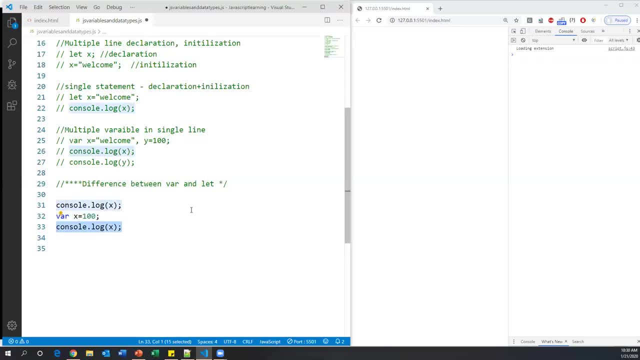 Then again I am printing the value. So if I save this file and see the console window, So what is an output of this? statement is undefined. And after that x value is become hundred, Then here hundred is printed in my console window. Perfectly fine. 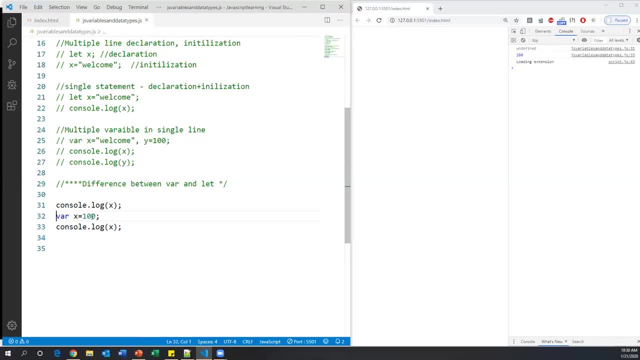 So instead of var, Because this var is function scope, So even x is not defined, So it is giving just undefined. But instead of var I will use let keyword. Then we will see what will happen. I will say let here. 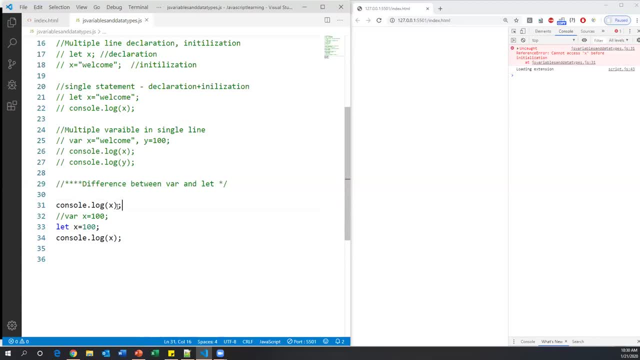 Now I am saving this. Now you can see the first statement is giving an error. So reference error: cannot access x before initialization. Cannot access x before initialization. So here x is initialized after printing the value of x. So this is not yet defined. 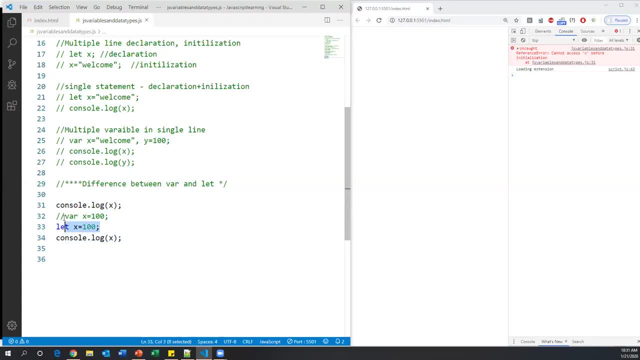 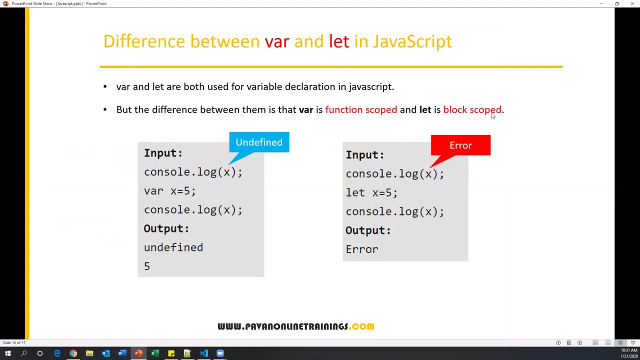 So we cannot access x before the declaration. But when I define the variable as var, We can access this variable value before the declaration. So this is the basic difference between var and let keyword. So var is a function scope Whereas let is a block scope. 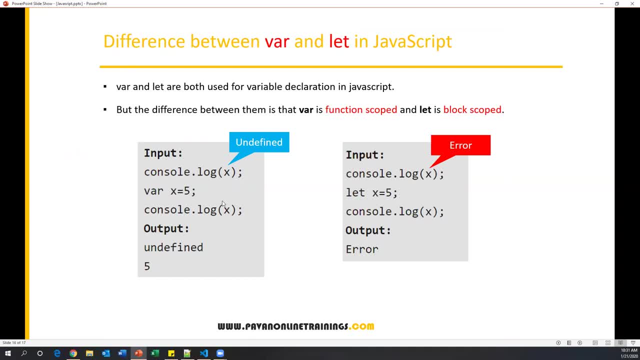 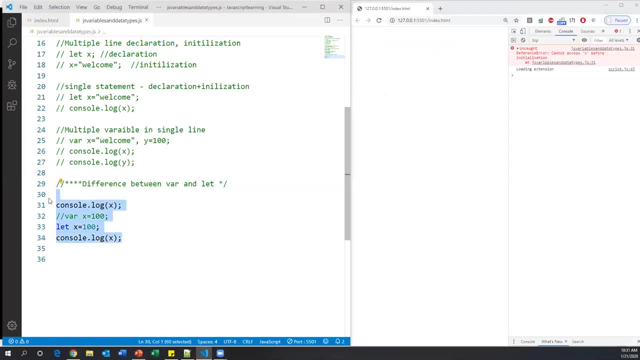 So this is the difference between var and let keyword. So, apart from these two keywords, We also have one more keyword called const keyword, So we can declare the variables by using const keyword. Now let us see where exactly we use const keyword. Let us comment this. 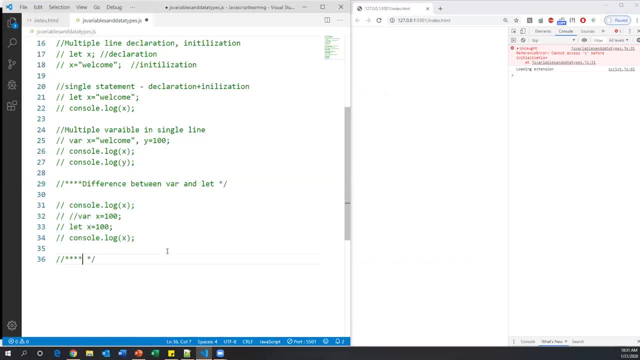 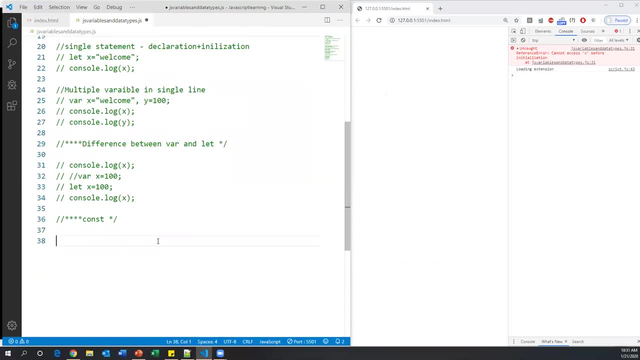 So how to declare the variables by using const keyword C-O-N-S-T. So to declare the variables by using const keyword, We have to use like this: So const, Let us say variable, Let us say x again, So we will make it as 100.. 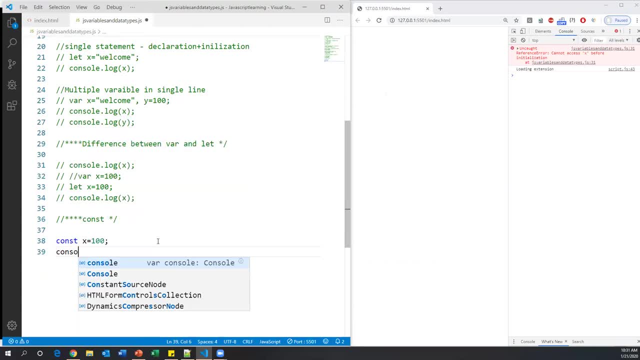 And then I will print this value by using consolelog, Consolelog and printing value of x And then semicolon Save it. Now we got the x value is 100. Perfectly fine, Right Suppose, after defining this variable I am trying to change the value. 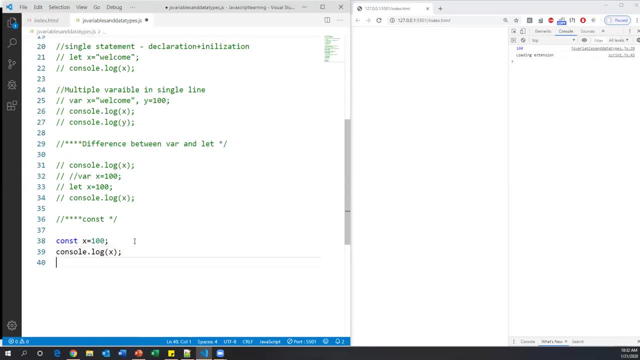 So here, after printing it Again, I am changing the value. So let us see here x is equal to. I will make it 500.. Right, So again I am trying to print it here. So two times I am printing. So first, x is equal to 100. 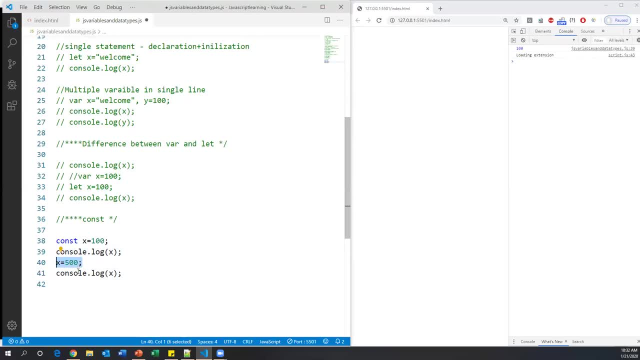 I am printed here And again I make it: x is equal to 500.. And then again I am trying to print here: Now save this. Now we got an error. So the first statement, x, is equal to 100. And we have logged that value here. 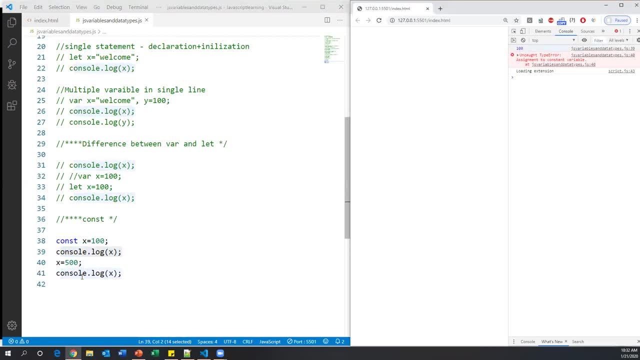 100 is printed in the console window, And after that I am trying to change the value of x. So then it got an error. So, uncaught type error. So assignment to the constant variable. So what does that mean? is This variable we have defined with a constant? 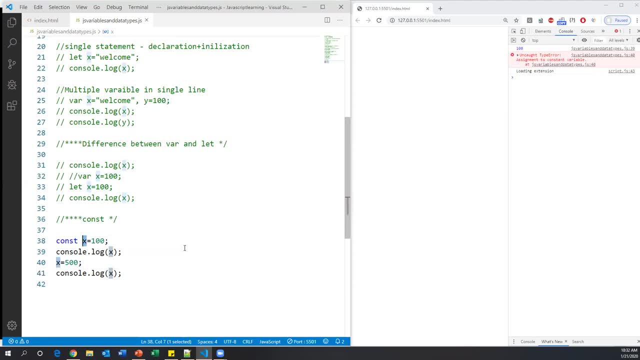 That means this variable value we cannot change. So once you specify this variable as a const keyword, That variable value is fixed. So we cannot change that value. But here we are trying to change the value. So this is incorrect. This is syntactically incorrect. 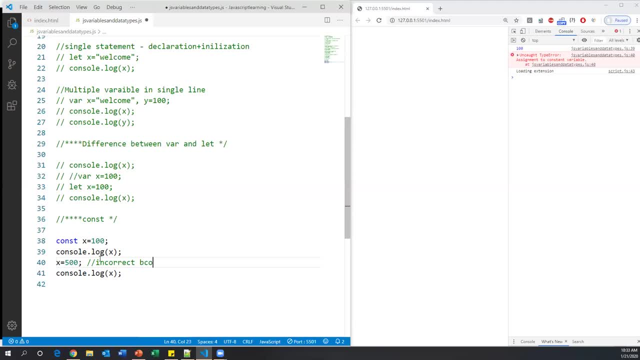 Because x is Because x is. x is const variable, x is const variable. So if you want to define any variable Which value should not be changed, Or if you don't want to change that value throughout the program, Make that variable as constant variable. 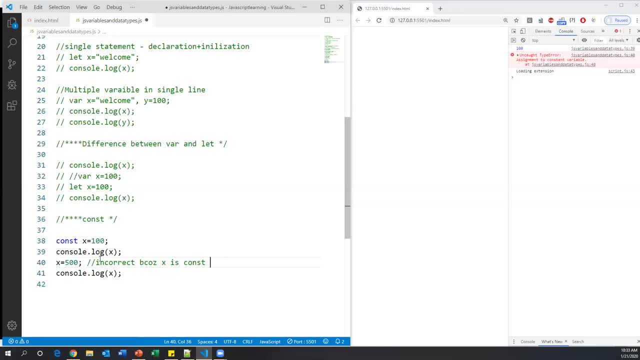 Constant. Where is const? C-O-N-S-T? So these are the different keywords available. So where is one keyword? Let is another keyword, Const is another keyword. So by using these three keywords We can define the variables in JavaScript. 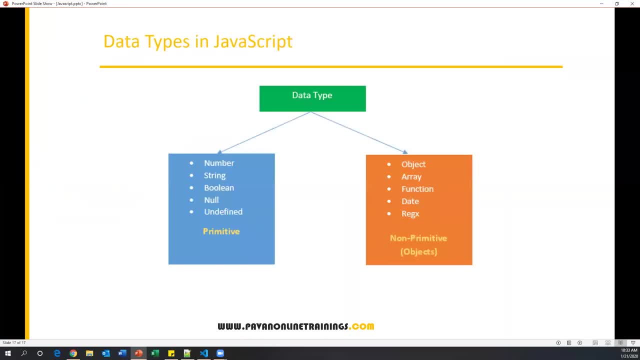 So now let us move on to the data types in JavaScript. So what is basically data type is? So every data which we have to represent depends on some data type. For example, I want to represent student number, student IDs, So they are basically numbers. or I want to store some prices of items, So they are decimal numbers. or I want to store the names of employees, So the data should be the stream, So that depends upon the data. There will be some corresponding data type in every programming language. The data types will be there. So data type is basically represent the type of data which we are going to store in a variables. 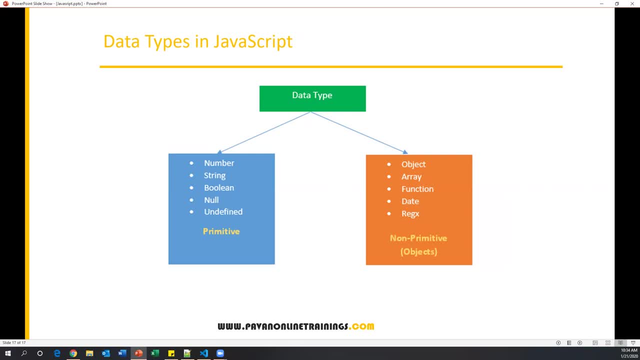 So normally, if you go for any other programming languages or Java or C, C++, we must define the data type of the variable before assigning the value. But in JavaScript we no need to specify the data type explicitly And what kind of data we are assigning to the variable. by default the data type will be associated or added to that variable. So what I'm, what I'm saying here is normally if you go for Java or C, C++, if you want to store in number, 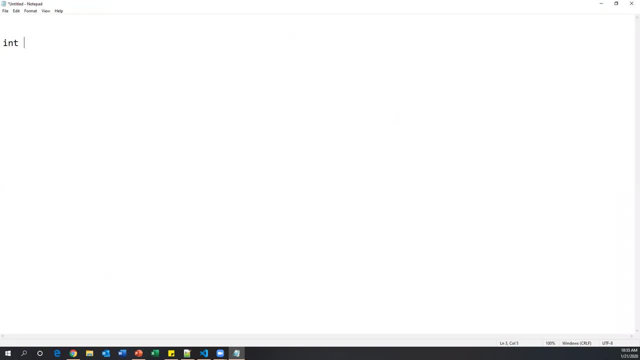 in a variable, you have to specify their data type. And then let's say: if it is ID, ID is a variable name. I can save like this: So here in these a data type, ID is a variable, 101 is a value. So in C, C++, Jawa, this notation will be followed, Especially in JavaScript. JavaScript is: 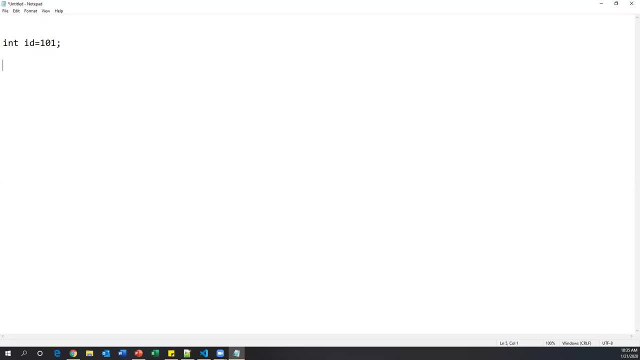 basically dynamically typed a language: JavaScript, basically dynamically typed a language. What does that mean is in JavaScript, We can directly write the variables like this: let us say where or ID is equal to 101. then what will happen is we no need to specify any data type? 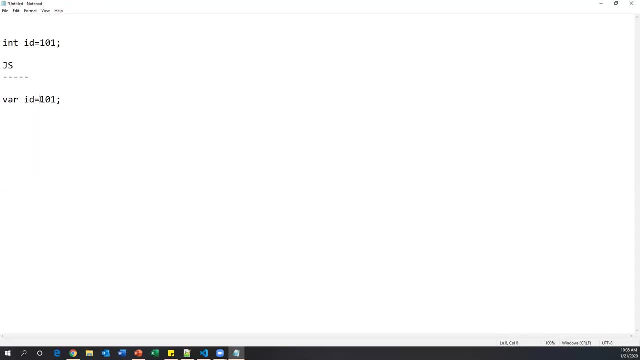 in front of this variable. so depends upon the type of data we are assigning to the variable. it will automatically consider the data type. so it will automatically consider this ID is a number, data type. and similarly, when I define a variable, let's say where name is equal to, I'll say John right, this is a 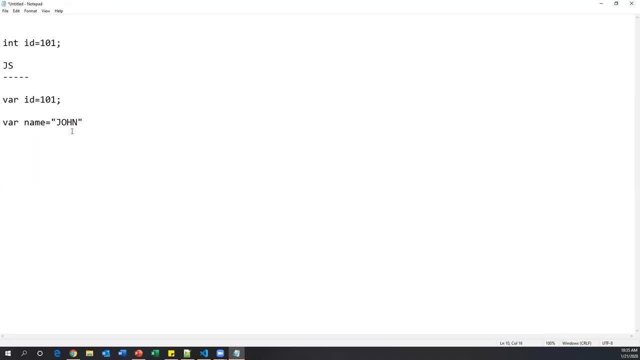 different type of data. this is a different type of data, so JavaScript automatically consider this name as a string data type, data string variable right. similarly, JavaScript is basically dynamically typed language. what is a dynamically typed language means we no need to specify the data type explicitly, so depends upon the data or type of data. it will automatically associate a data. 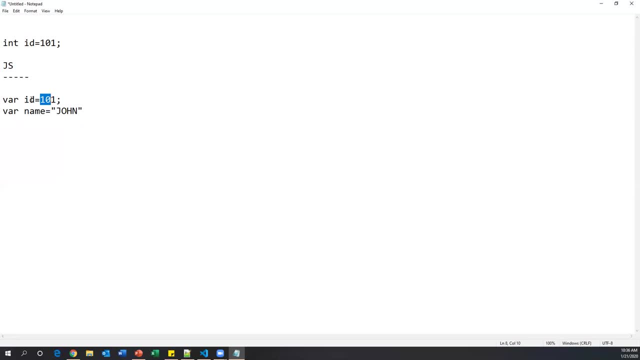 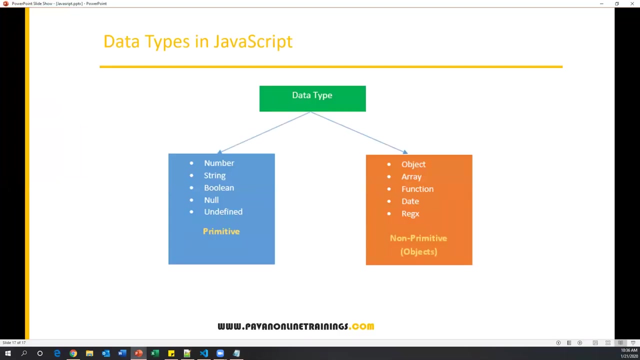 type to that variable. that is called as dynamically typed language. this is a feature which we have in JavaScript. okay, so now we'll see how we can work with the data type. so what are the data types are available. so in Java we have a number, string, boolean, null and defined. so 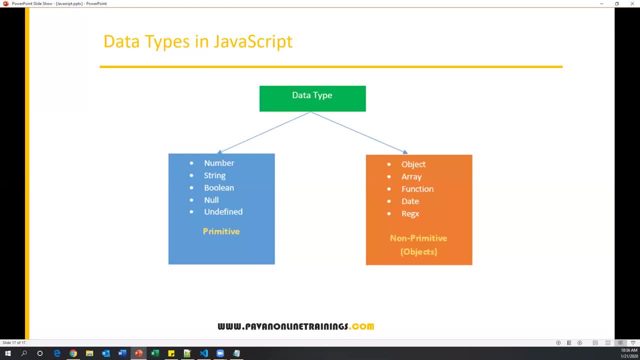 these five are called primitive data types: number, string, boolean, null and different. so these are all primitive data types. apart from this, we also have non-primitive data types, or we can also call as objects, like object array function, date ring X. so these are all the different object type data types. so 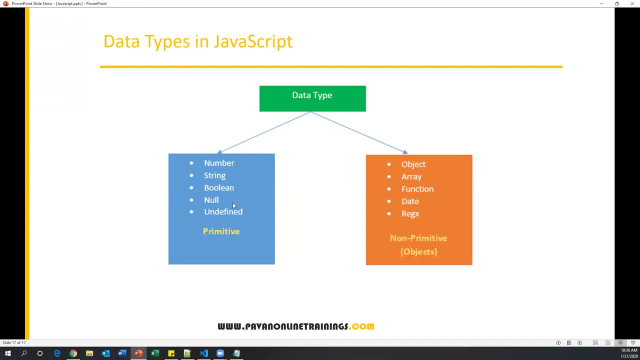 we will. we will see them in the coming session. so far now i will discuss about primitive data types: number, string, boolean, null, undefined. so, as i said before, we no need to specify the data type in front of the variable at the time of declaration, because javascript is a dynamically typed language, depends upon the data or type of. 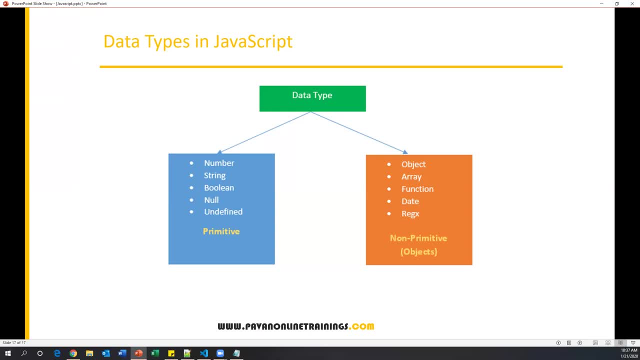 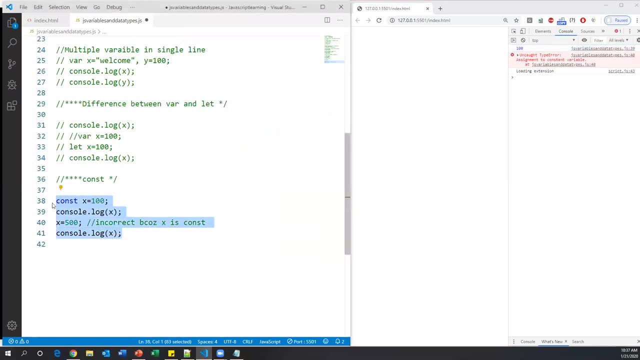 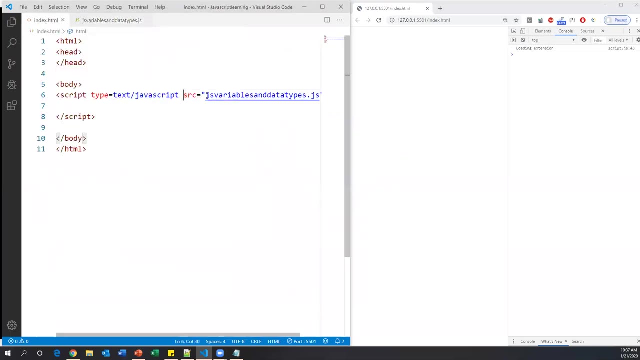 data. it will automatically assign the data type to the variable. now we'll see if. one example, few examples. let's go back to javascript here. i'll comment this. all right, so now save it. so just remember, this javascript file is already referring in our html, so currently our html file is running. 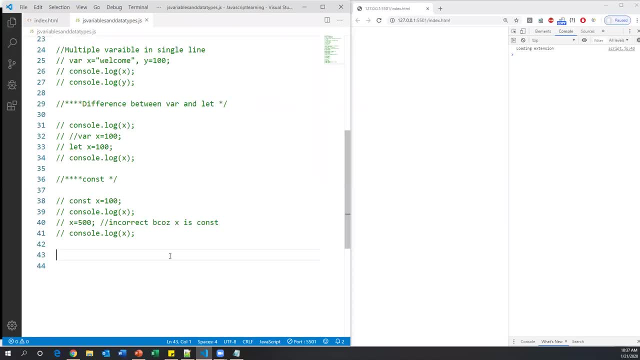 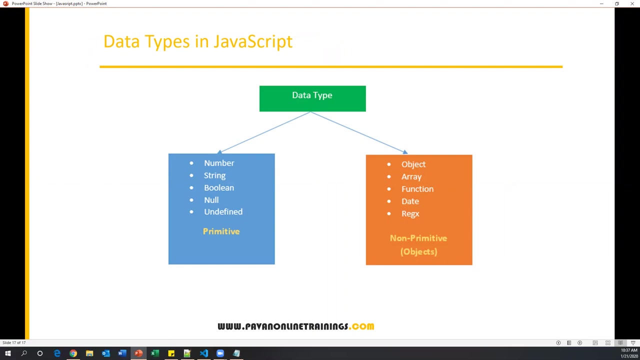 on my live server. okay, so now let's go back to the javascript file, and here i'm talking about data types. data types, right, so data types. so what are the data types available? so, as i said, we have number, string, boolean, null, undefined, and also, we have seen, javascript is a dynamically typed language. 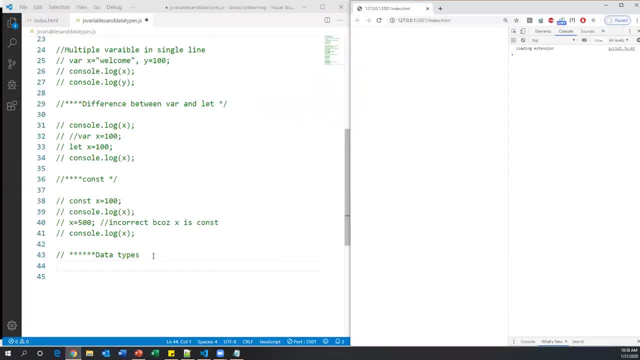 i will see how this feature is going to work. so i am defining a few variables. let's say i'm using let keyword to define the variables, let x equal to, let's say, 100. so i have defined a variable called x and i have assigned some data to the x, and this particular data is basically a number. 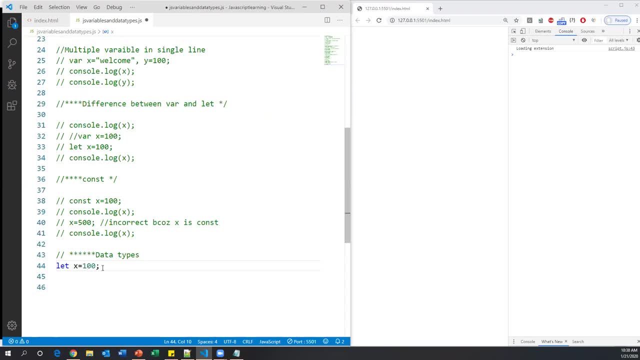 type right. so numbers- it can be integer or decimal- will be considered as a number type in javascript. but how we will know that? so i want to know exactly what kind of data, what kind of data type is assigned to this x. so if you want to know that we have, a special method is available. 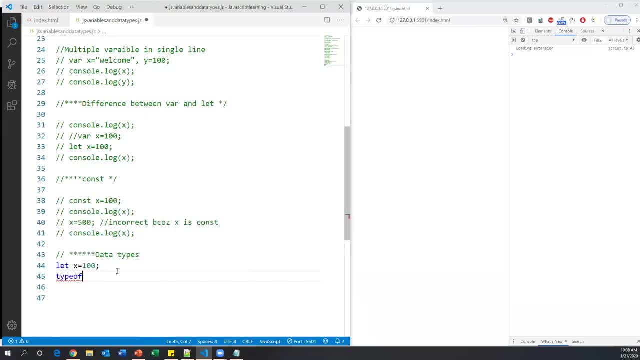 that is called typof. so when i use this typof type of x, this will basically return the data type of this x. but here we don't know exactly what is this x제yор kusliyor. i don't know exactly why. i didn't know this. 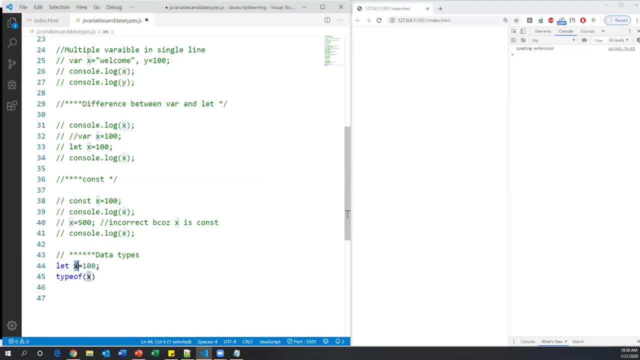 exactly what data type is associated with this x. but if you want to know that i have type of x type of method will give you what is the data type which is assigned to this x and that return value. how to print right? so i'm just printing the console window. so console dot log. type of x and. 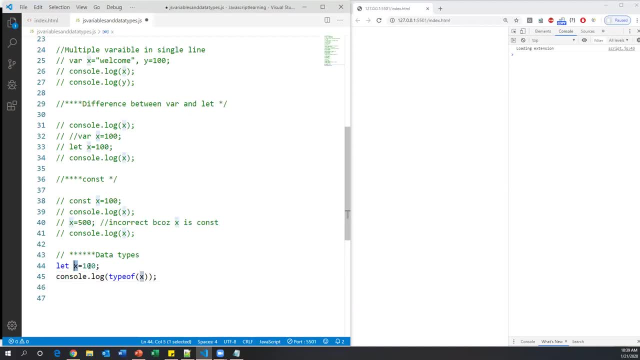 this will give you exactly the type of x. depends upon the data. now save it. now you can see on the live server it is written number. so this is written number, is a data type. because we already added number and suppose i'll say, let x is equal to less, x is equal to, or i can save a different. 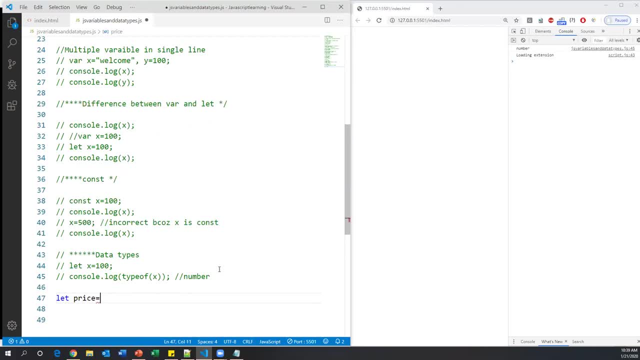 number. let's say let price. price is normally in the decimal format, right? so let's say 100.50, so this is decimal number. this is also number type. let's print here the type: so console dot, log, and i'll say: type of so type of price, type of price. now, even though this is decimal number, this is also number. 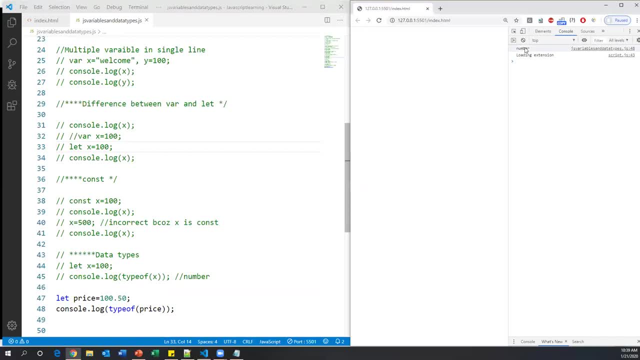 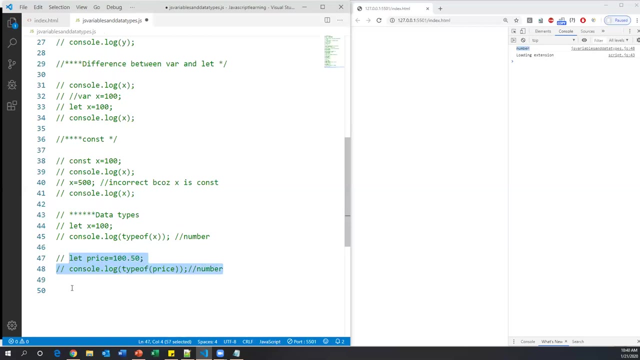 so let's save. and now you can see this is also number. it is also written as a number, perfectly fine. so integers and decimals, both will be considered as a number data type in javascript, right? so now we'll see other data types. suppose i want to store a student name in a variable. 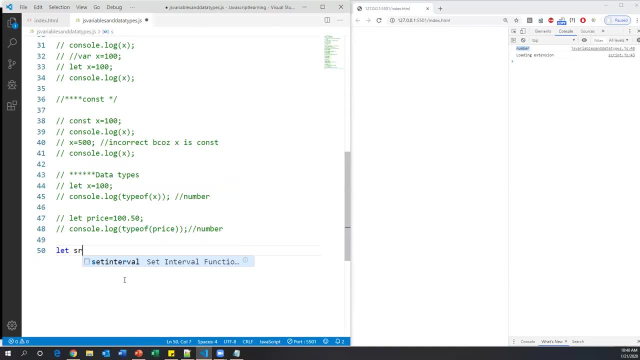 so let's say i want to store a student name in a variable. so let's say i want to store a student, let let stu name, equal to it is a student name, should put in the double quotations because this is a string. so stu name, i'll say student m a m e. student name equal to, i'll say john. 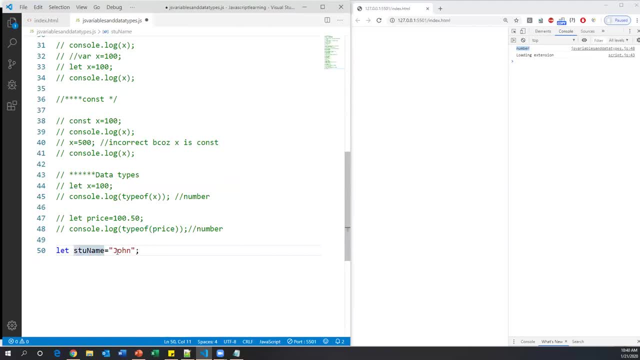 okay, so this is a string type of data, so we'll see what kind of data type is associated with this variable. so to do this again, we have to use type of type of stu name and this will return the type of the variable. then let's print it so: console dot log. type of stu. 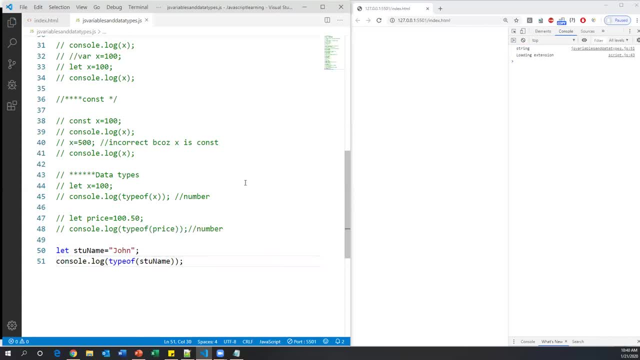 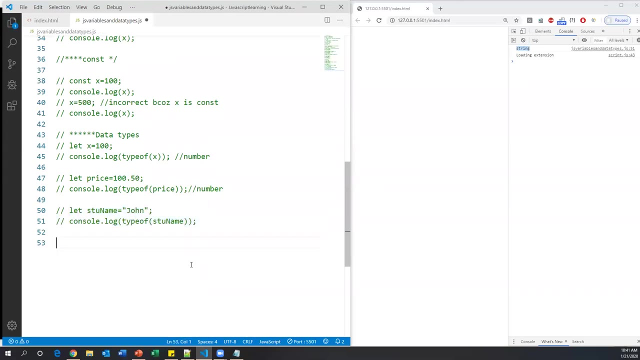 name, then semicolon. now save this. now you can see here it is written string. so javascript by default associated the data type to this vehicle based upon the data we have assigned. now, similarly, let us see another data types. let me just comment this. let's say let, uh, let let's say flag. 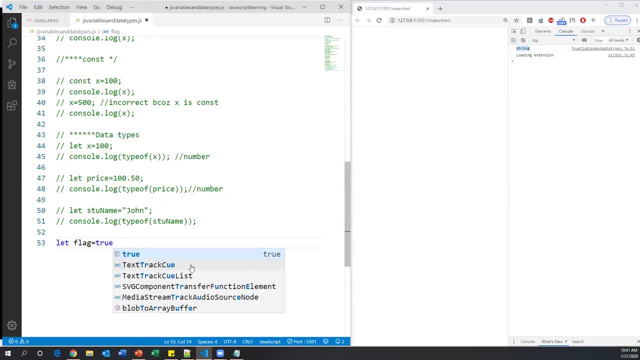 is equal to, let's say, true. so this is a boolean type of data. we can assign either true or false in lowercase letters. now if you want to see what kind of data type it is, we'll say console dot, console dot, log, and here again type of type of flag. so type of flag and semicolon. now we can refresh and 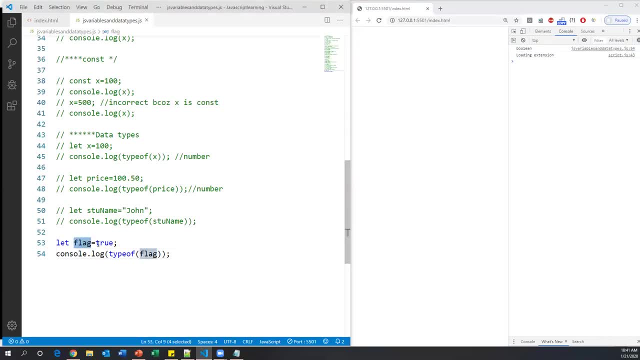 save. you can see boolean, so this flag is considered as a boolean. now i can also say false. false is also a boolean value. now save it. you can see still boolean, so this will consider as boolean data type if i assign either true or false. and similarly we also have other data type called null. so for 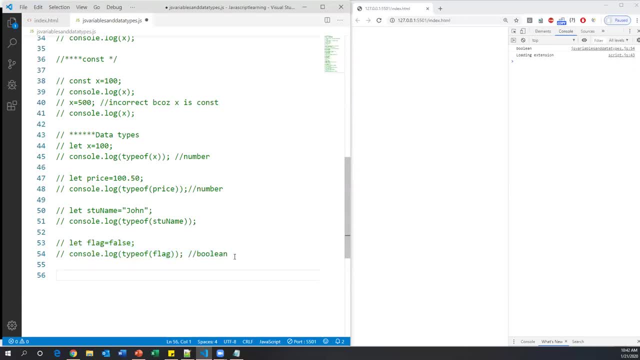 example. let's say so, let's say let, uh, let let's say status. let me take a status equal to null. so null is also another type, data type. so let's say null. and then let's print: so console dot, console dot, log, and again type of type of status. now i'll see, refresh it and save and you can see. 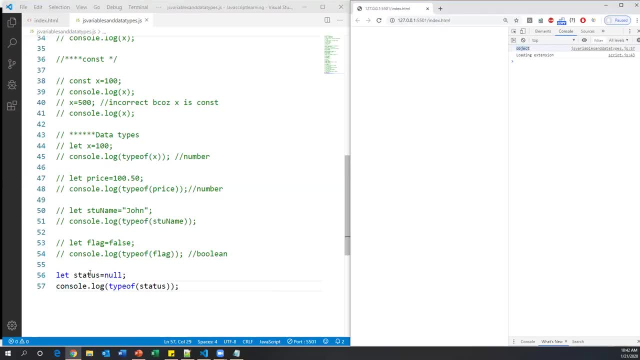 it is returning object. so when i say, when i assign null to the variable, that will be considered as an object type, object is also one of the data type in javascript. so here, when i assign the null to the variable, that will be consider as a object type, object type. and apart from this, we also: 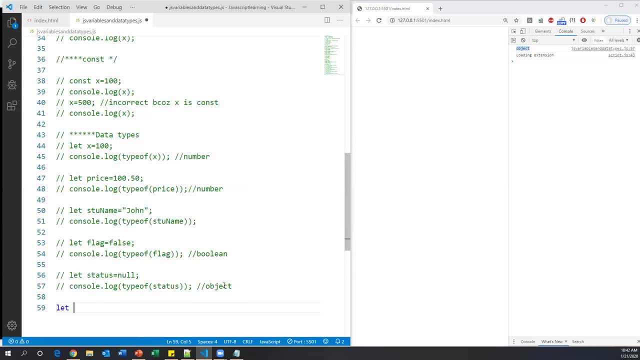 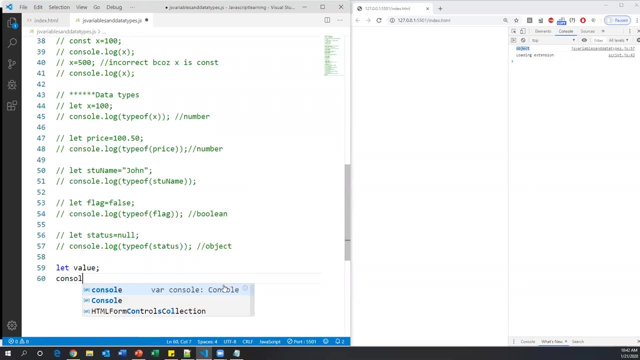 have one more time available, so called undefined. let's create a letter. value is equal to. i don't specifying any value, just define the variable and try to print that value. let's say console dot log and let's say type of type of value: type of value. now you can see here: i have not assigned any value to this variable. 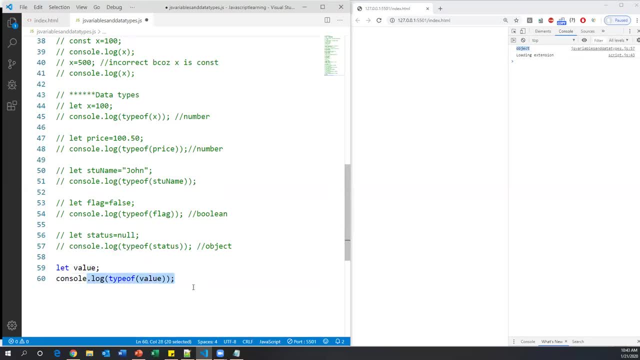 right, just let's let value and then i am printing the type of value. now we'll see what kind of value will be assigned by default. so let's save it and you can see. in output you can see undefined. so undefined means i haven't assigned any value into this variable. so 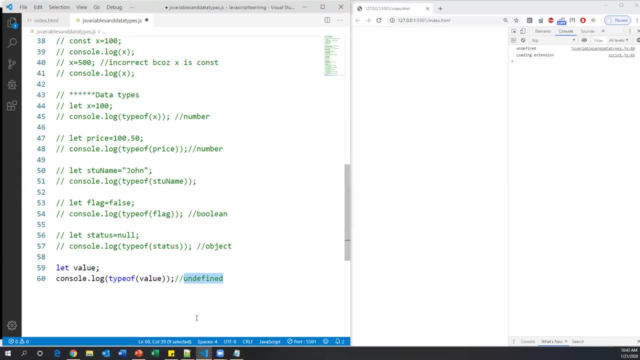 that's the reason javascript will be assigned undefined. type undefined. so suppose, for example, you can also directly assign undefined. here you can say undefined. this is also type of data. so when i say undefined assigned to the value, obviously this is also undefined. save it, and now you can see it is still showing undefined. okay so, but what is the difference between null? 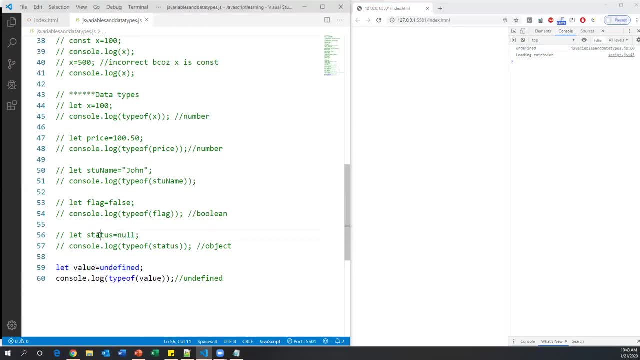 and undefined here. so when i assign null to the variable, that variable will be considered as an object type, whereas when you assign undefined to the variable or if i don't assign any value to the variable and that variable will be considered as undefined type. so here this: 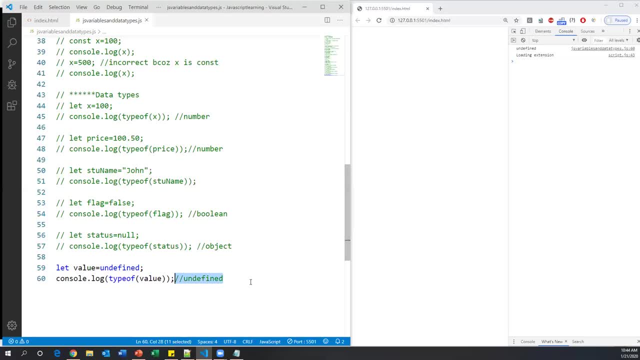 is object type and this is undefined type. these two are the different data types in javascript. okay, so is a difference between null and undefined. so null is basically an object. if i assign a null to the variable, that will be considered as an object, and if i don't assign any value to the